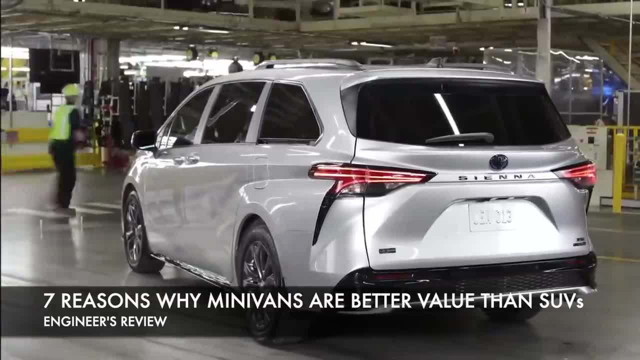 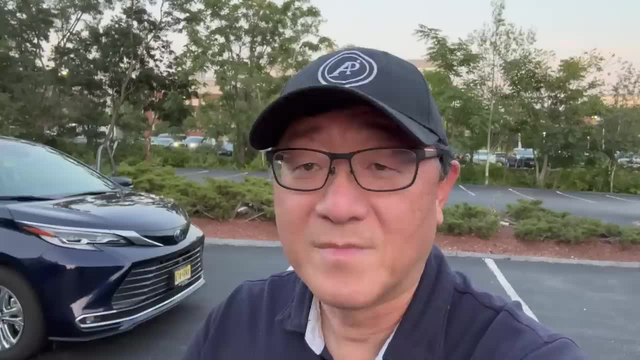 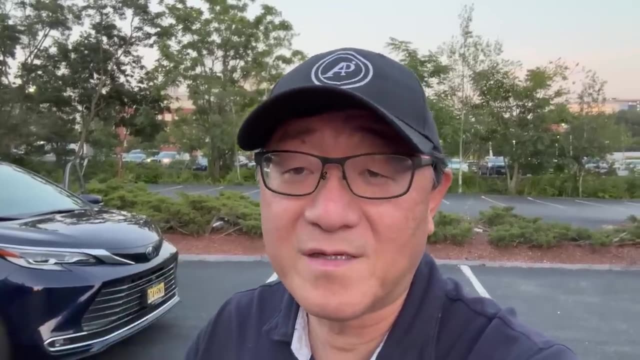 reasons why I believe minivans are still good and perhaps better buy and a better value than SUVs. Let's go Welcome back. By the way, I'm in Boston here, which is kind of interesting because, as some of you guys know, I actually went to school in Boston for my postgraduate studies. 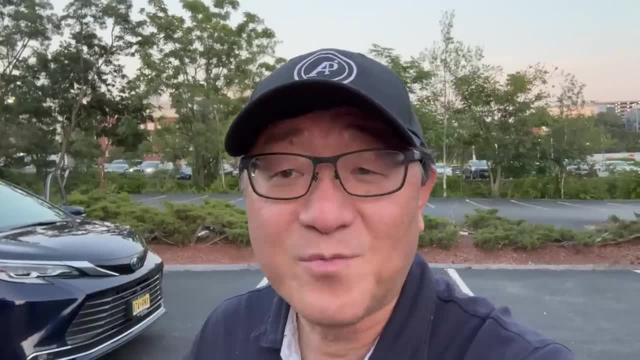 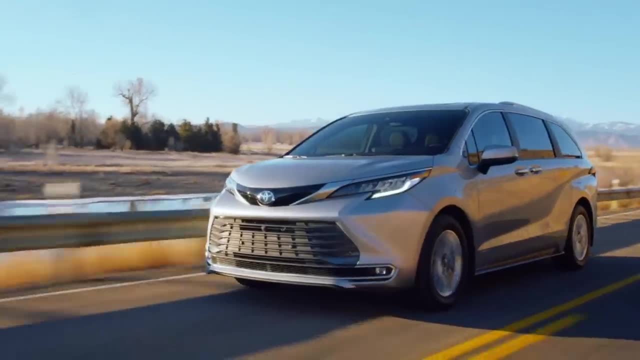 because I studied at MIT and Harvard and I was kind of coming back to my third home- not quite second home, Because I consider Toronto to be my second home, where I spent many years as well. Anyhow, I want to walk you through seven reasons why I actually think minivans in general, especially. 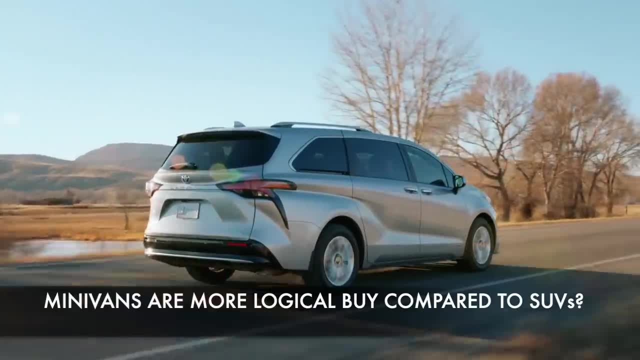 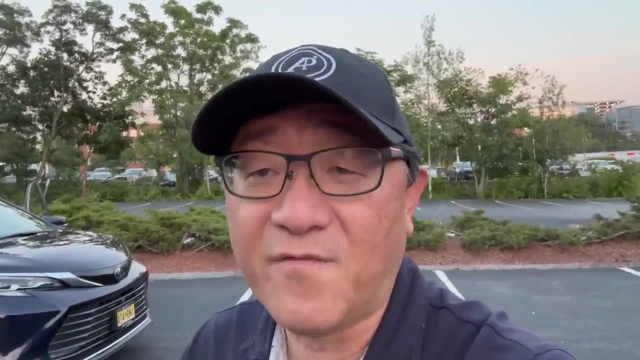 this Sienna here is a better buy and a more logical choice than sport utility vehicles and crossovers, because they just don't offer the same amount of practicality and functionality. So let's start with the first one, which is all to do with how the minivans are designed. 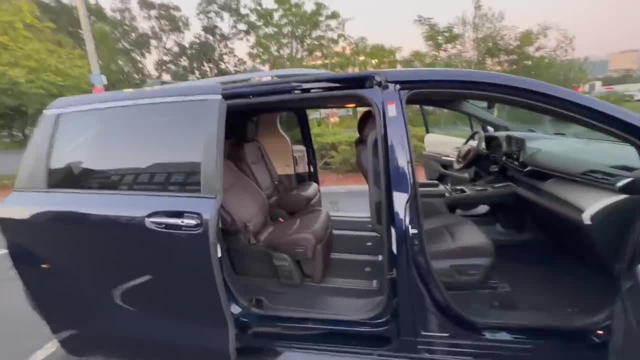 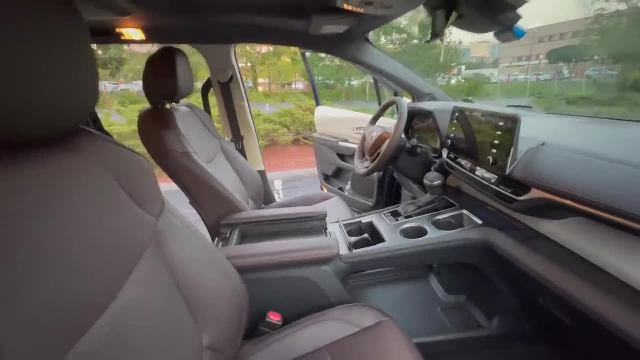 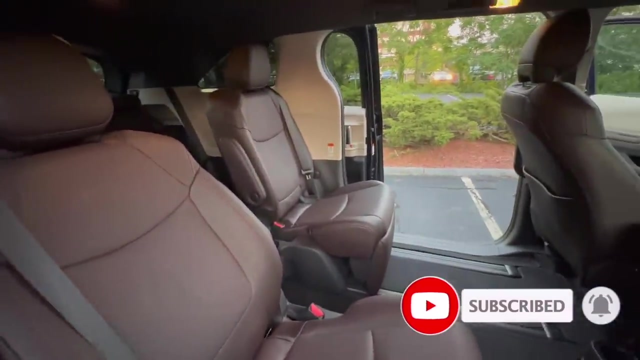 Because of the way the body is shaped and profiled and because of the way they design the interior, you get maximum utilization. There's nothing out there that can match the minivan in terms of the overall space, overall efficiency and packaging. Look at how much space we have here. Obviously, 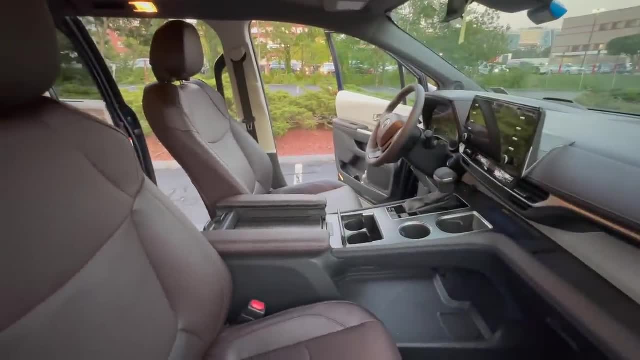 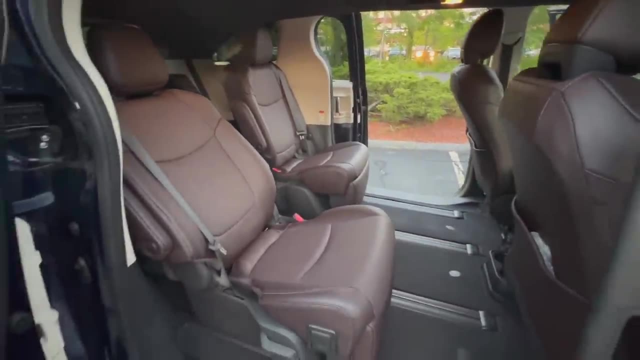 the front row is very good, but maybe it's comparable to a large SUV. But when you get to the second and the third row, that's where the big differences are. This is almost like a first class cabin in an aircraft. here These seats can recline. We can also pull up the leg out here. 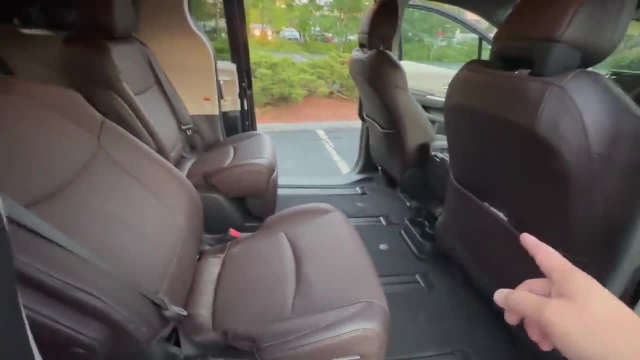 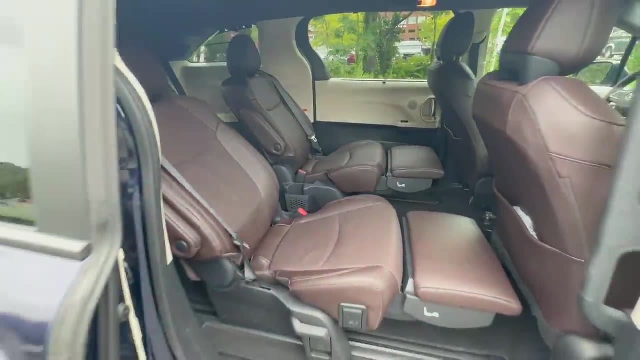 As well, which I'll show you a little bit later. And look how much space there is between the first row and the second row. There's just tremendous amount of space and it's an extremely comfortable environment. And you know what? It's not just about the passenger space, It's also about the 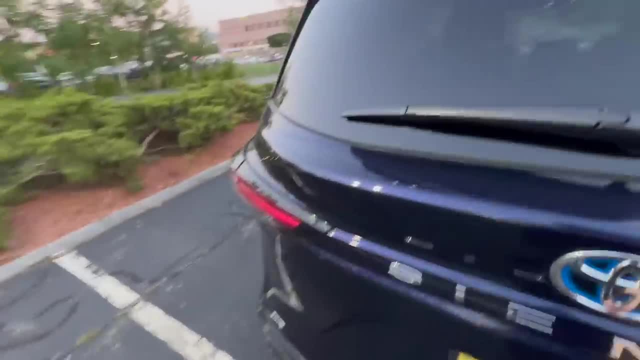 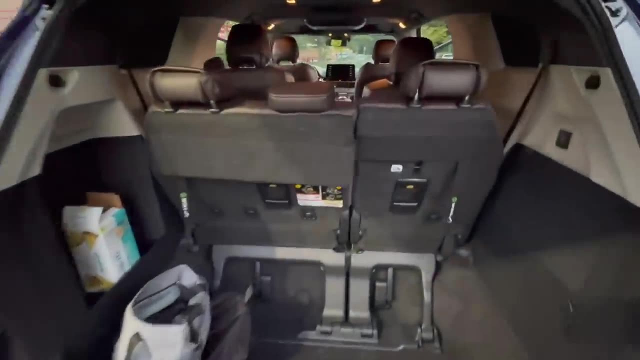 trunk space as well. So I'm going to open the back here and show you what I mean by that, because there's just so much cargo space Now. right now I have the third seat up and you can tell it's pretty reasonable space, Maybe a little bit tight in the leg room, but it's not too tight. So I'm going to. 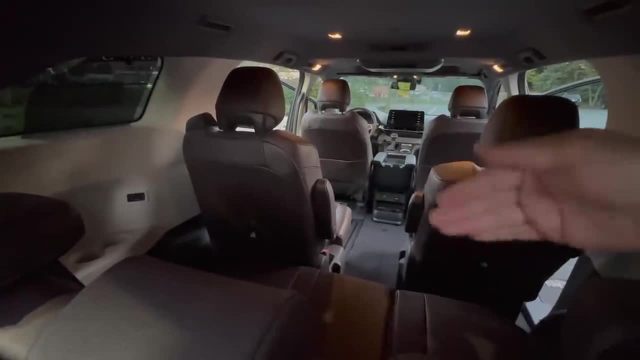 show you what I mean by that. Maybe a little bit tight in the leg room, but it's not too tight, So I'm going to there. But once again, those two seats are pushed all the way back right now. Once I push those, 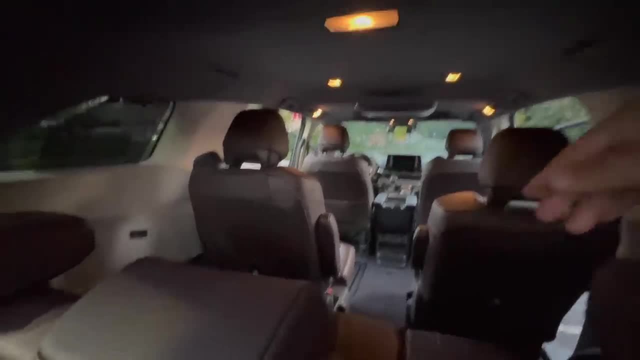 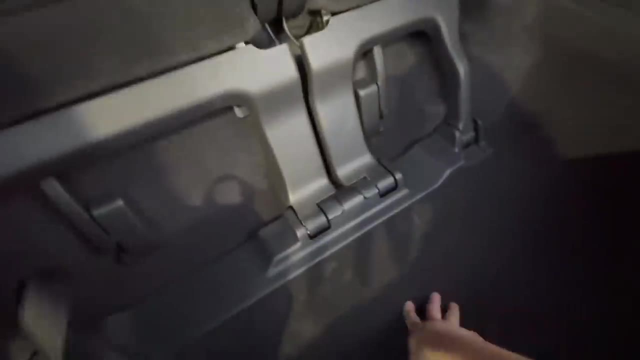 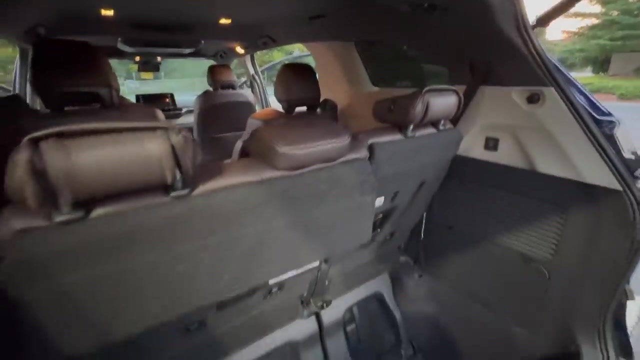 forward, you get a decent amount of a third row space, including lots of headroom. But look at the trunk space here. I don't have too much stuff in here right now, but look how deep it is. It goes all the way down here and then you can put stuff all the way to the roof line. So this space is. 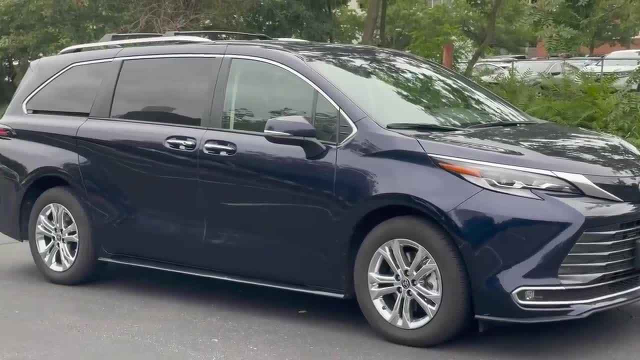 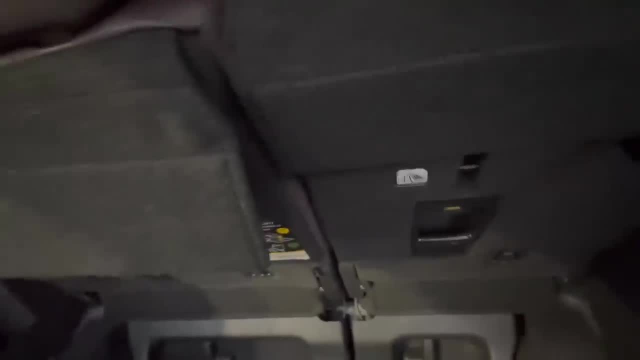 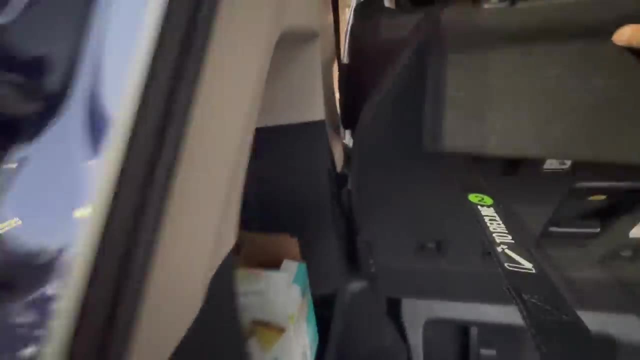 just a far cry from anything else that's in the sport utility vehicle or crossover category. Obviously, these things fall down as well, So let's just pull this up and see if I can do this kind of live, And let me pull this one as well. Oops, I can't quite pull down the seats right now. 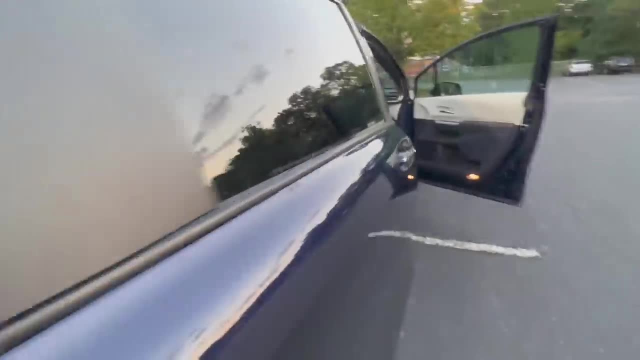 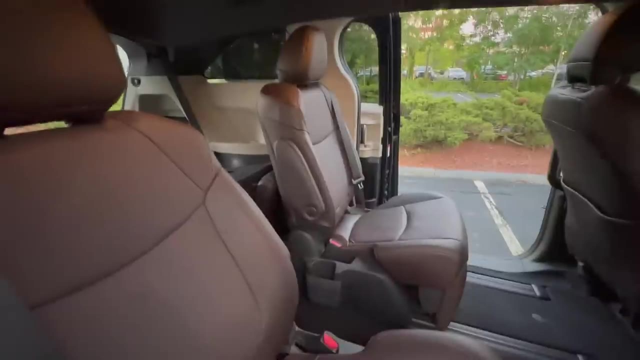 because I have the front two row seats pushed all the way back. So I'm kind of doing this live stream style. So let me push these seats forward and let's see what we can do. So I just moved these two seats a little bit forward. Still lots of space between front row and the second. 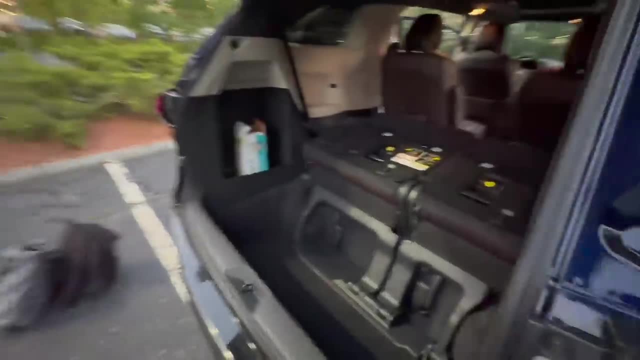 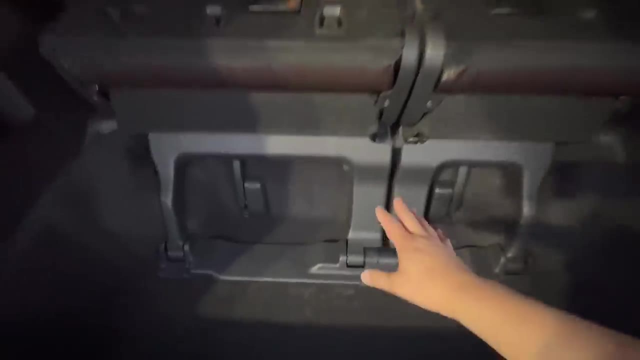 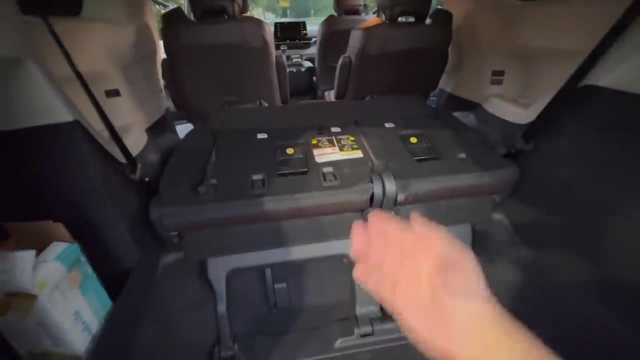 row, But I was able to move it so that I can actually fold down the third row And if I don't tumble this inward, I still get this deep, deep amount of cargo space that goes all the way to the floor here right to the top. But now I can tumble these seats backward and then hide them. 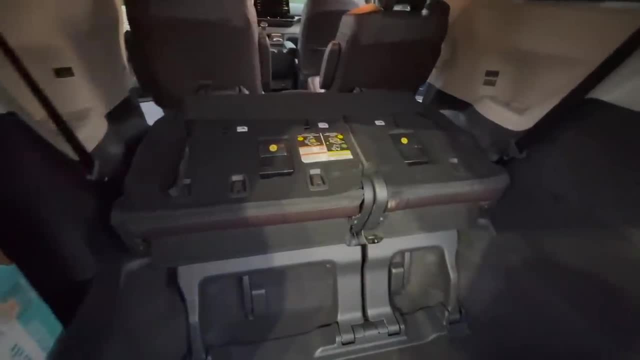 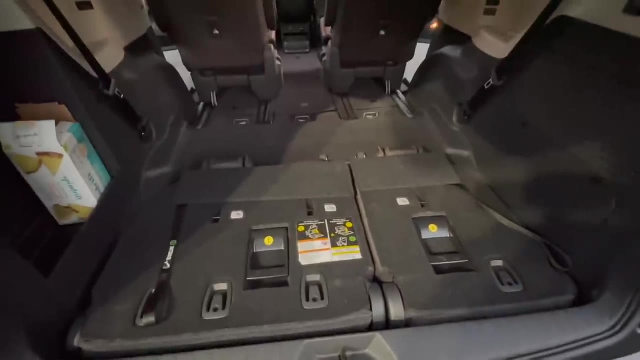 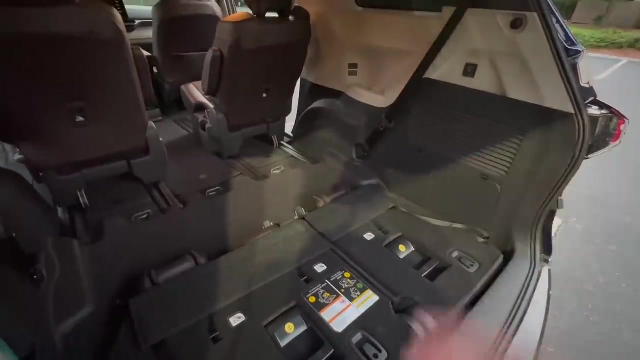 into the cargo area, And that way you get a flat seat. So let me do that right now, So I can just push them back like this. Still, both seats like this, And now I have a pretty well flat floor and look how much space I have. Enough to, you know, move a house or two. 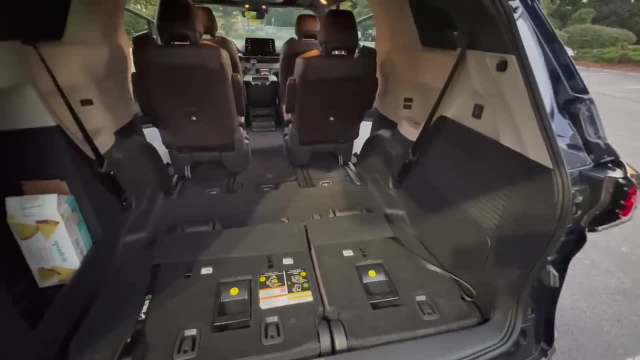 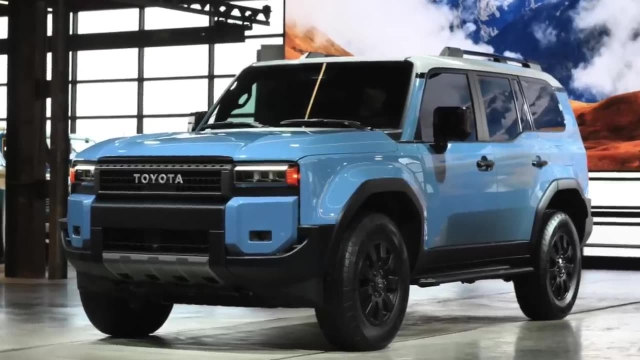 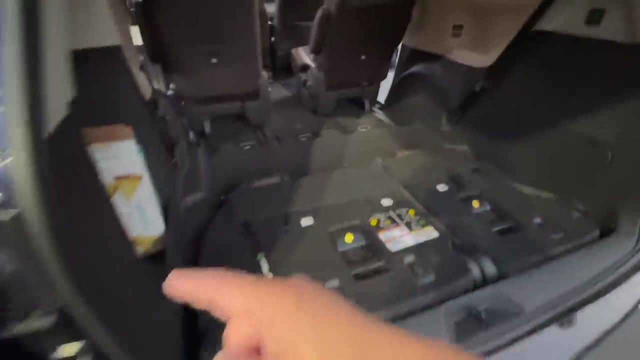 And that's something that today's SUVs are not very good, especially if they're body on the frame, such as the Toyota Sequoia or maybe even the new Land Cruiser. Any of the models with body on the frame design will have these floor much higher because there's a frame underneath which eats. 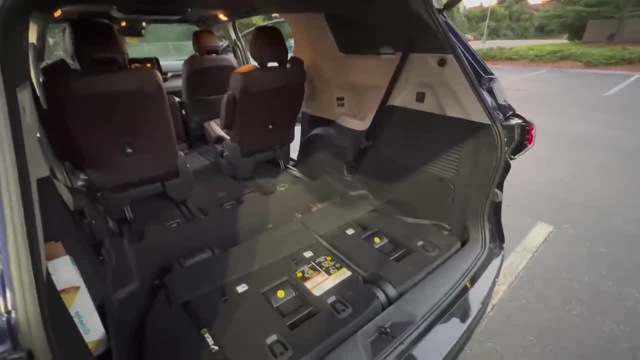 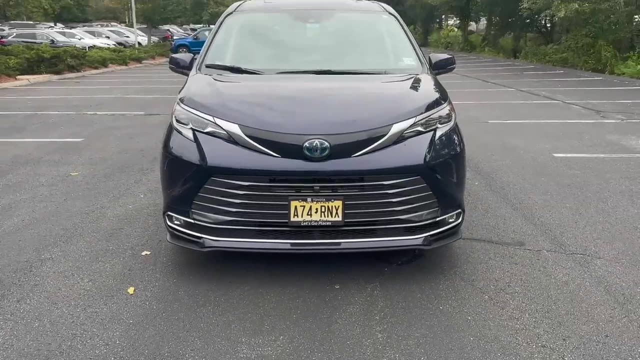 up the space. And it's worse if you have a hybrid Where there's additional battery pack underneath, as we have seen Sequoia. So, once again, in terms of space utilization, nothing can beat the minivan, both in terms of cargo space as well as space for. 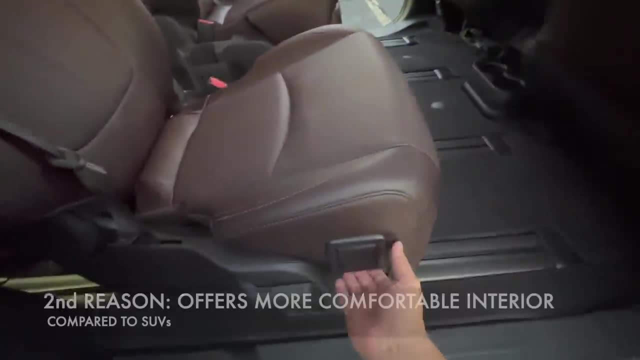 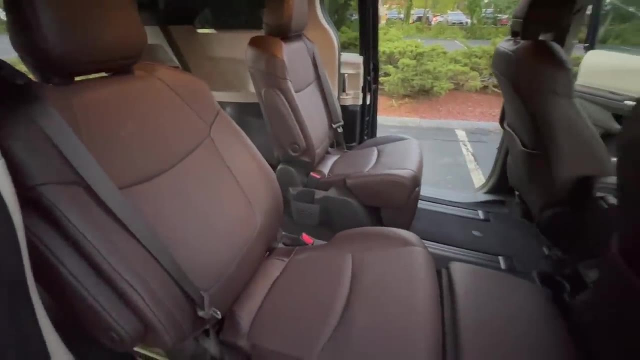 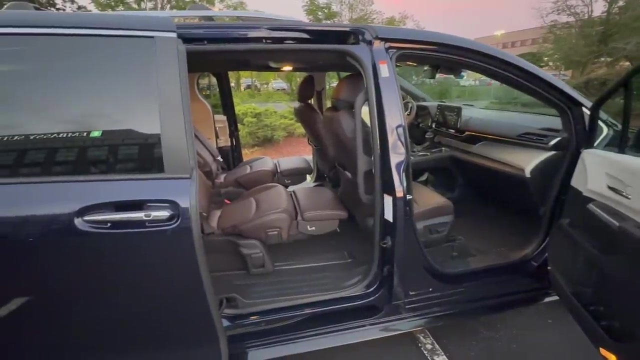 the second row of people And you can see, for example, here I can bring up the auto man style seat and basically almost fall flat. Not quite, but it's very comfortable And practicality. nothing beats minivans. The reason why minivans are superior to crossovers and sport utility vehicles is the fact that we get 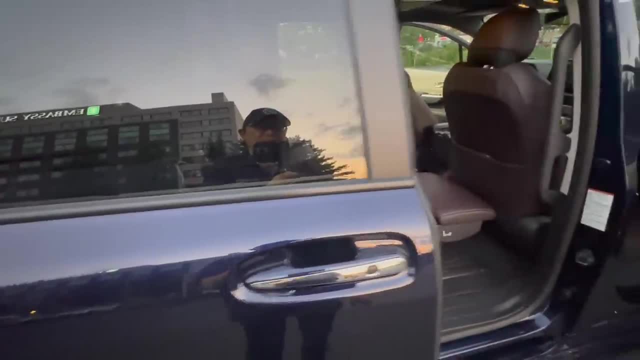 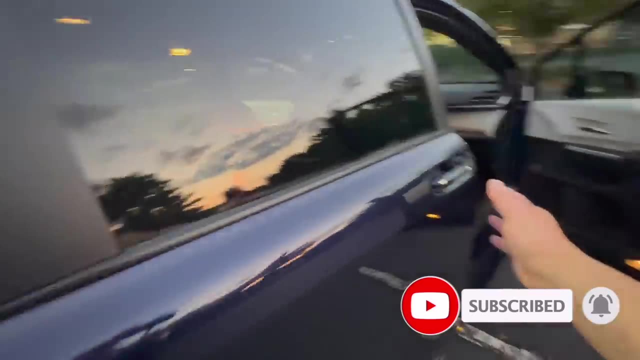 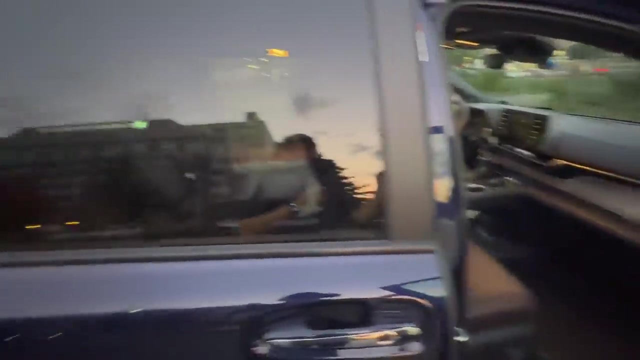 this sliding door, which is usually powered, so that I just have to touch the door and it will close. And you know what? This way, the sliding door stays close to the body. It doesn't swing open like the front door, So it's easier to get in and out in the parking space. And, as you know, 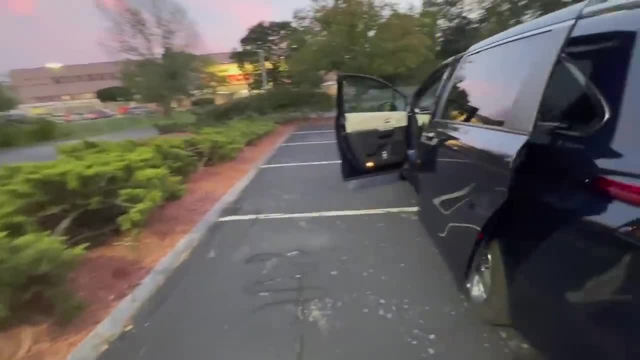 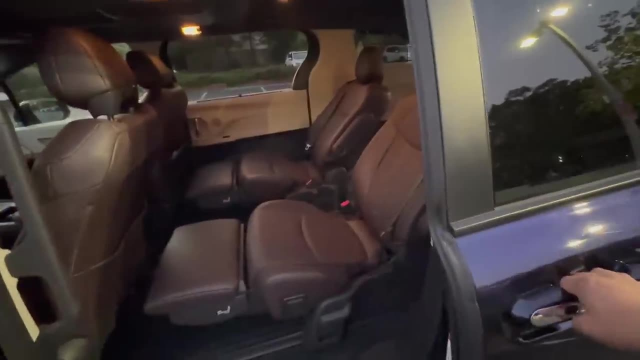 sport utility vehicles do not offer that. The only one that offers that is the new century SUV that was just shown recently, And they show sliding door as one option. But having this sliding door makes a huge difference in terms of getting in and out of the vehicle. And, once again, 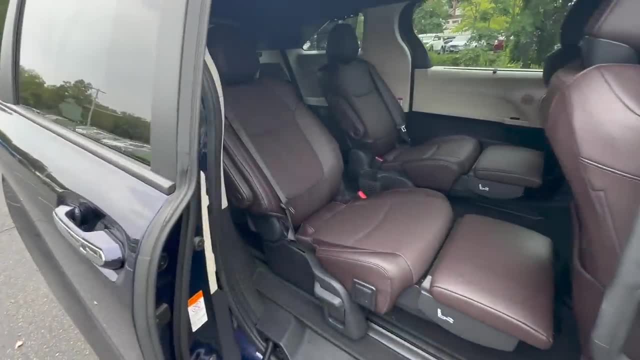 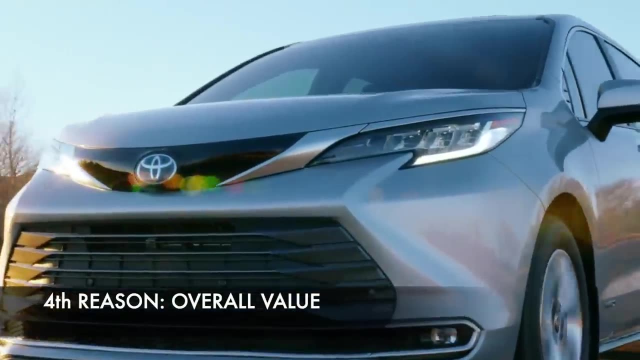 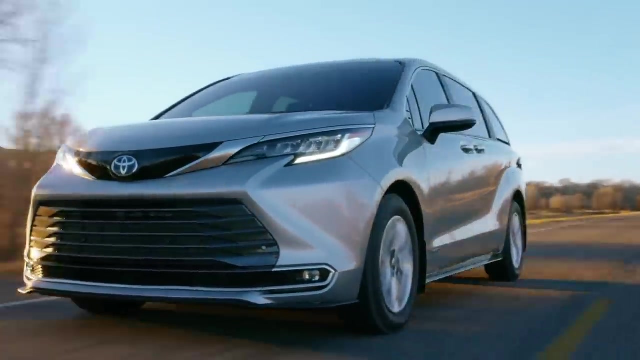 minivan trumps SUVs for ease of entry and exit because of the sliding door. The fourth reason is to do with the value Overall, pound for pound, kilogram for kilogram. the minivans are cheaper, sometimes substantially cheaper, than sport utility vehicles and 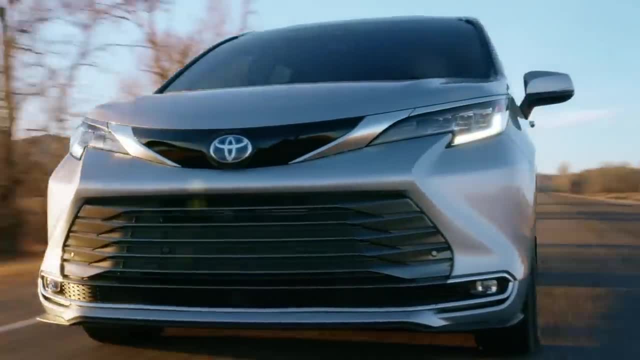 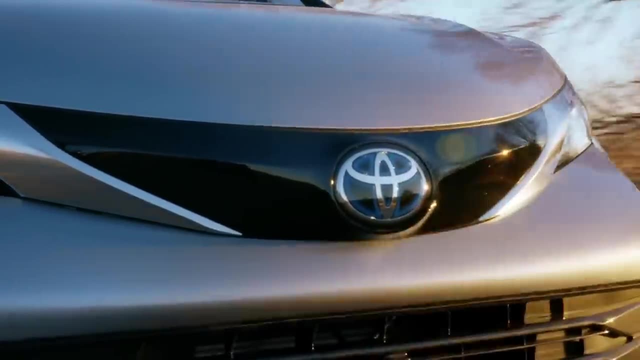 crossovers that offer similar space inside, And this Sienna, of course, is quite reasonably priced. Even fully equipped is way cheaper than something like a Toyota Sequoia, which doesn't offer as much practicality. So even though people are not too crazy about buying minivans, just 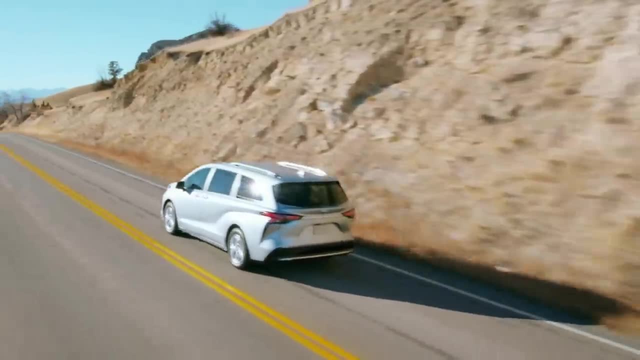 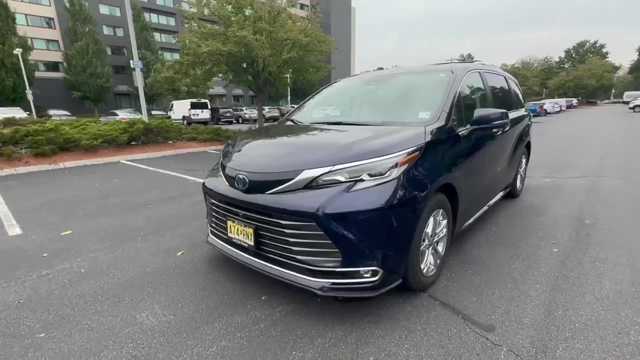 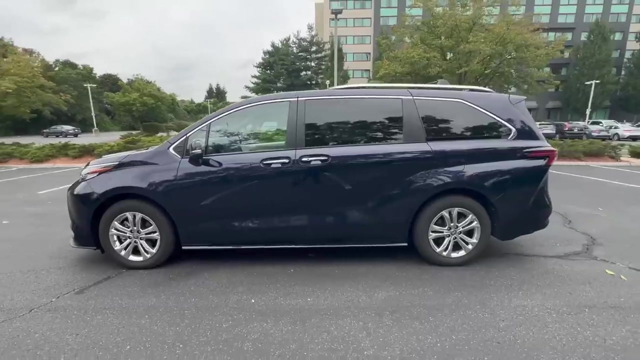 because of the type of branding they represent. you know what, if we can throw that away for a second and don't even think about the name minivan? definitely this is the better value. The fifth reason is to do with efficiency, Because minivans are definitely more efficient than equivalent sized SUV, especially if they're 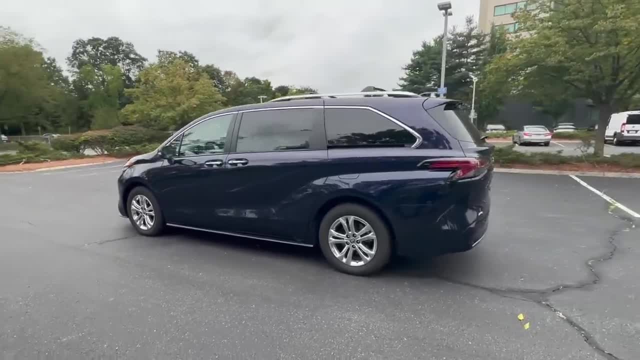 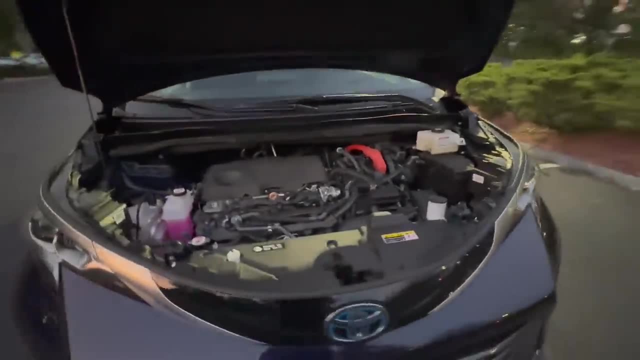 body on the frame. The Sienna has a hybrid system as well, And, even though it's not super fast in terms of acceleration, it's more than enough to go around town and pass cars on the highway. But, more evidently, it is extremely efficient, And because it is lighter, due to the fact that 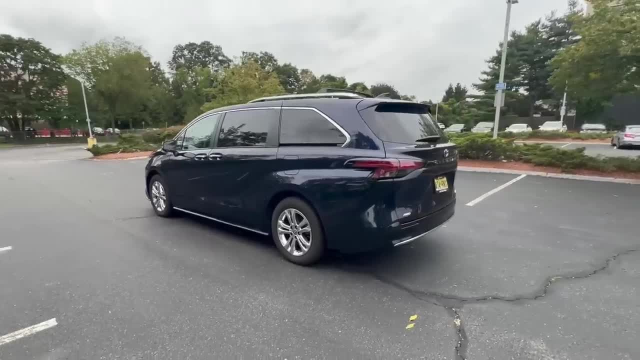 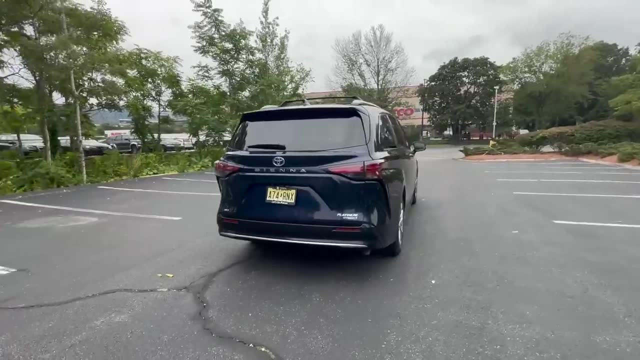 it's a unitized body compared to body on frame models such as a Sequoia, you just get overall better efficiency And if you want to save some gas, just have a better value and also save fuel, well, definitely minivans are better than bigger export utility vehicles. 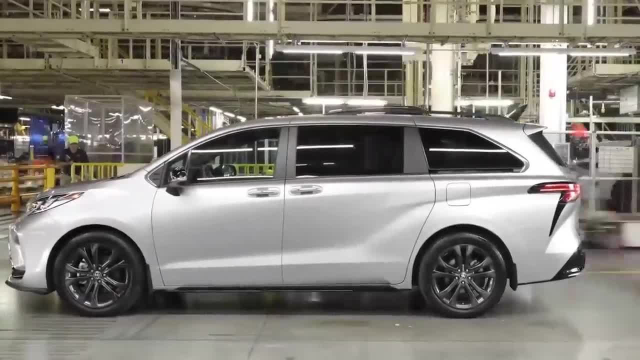 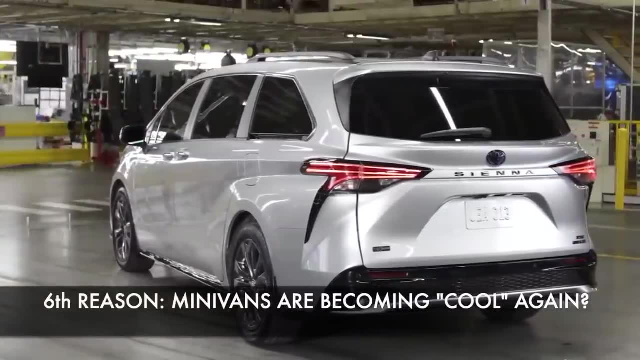 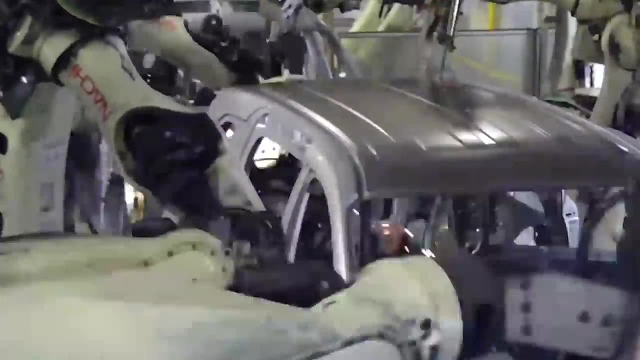 The sixth reason why I really do like minivans is something that's a little bit different than what you might expect, And that is to do with the cool factor, which you might be surprised, because no one thinks minivans are cool, But there is a bit of a resurgence in terms of the branding of minivans because in many 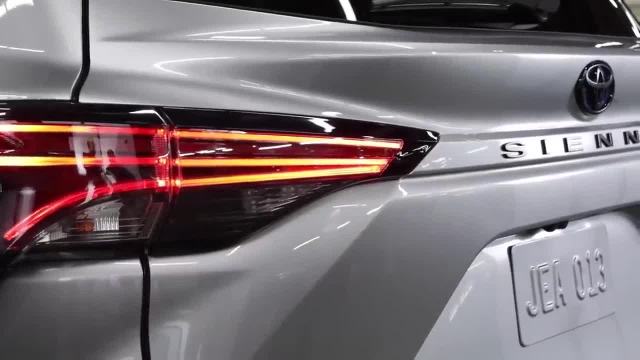 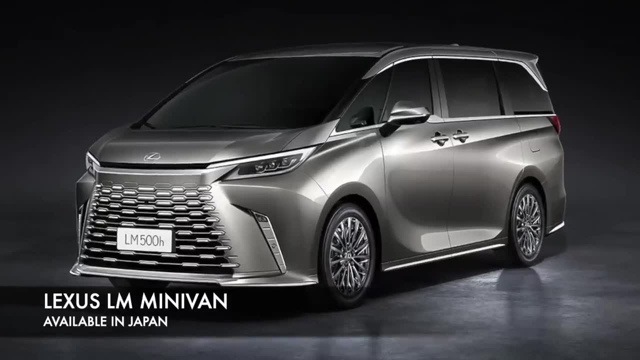 parts of China and Asia, minivans are definitely considered cool, especially as a luxury people mover, And cars like the Lexus LM, which was introduced recently, is showcasing how good minivans can be and how desirable it could be as a people mover. 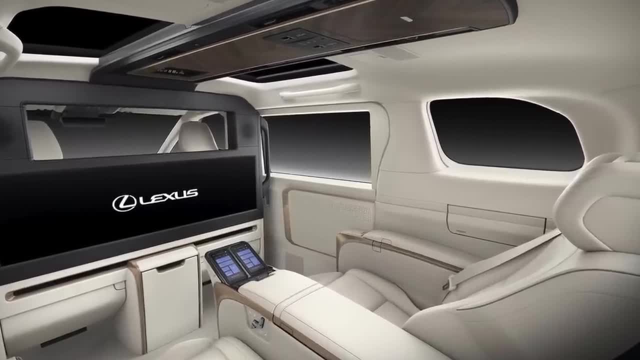 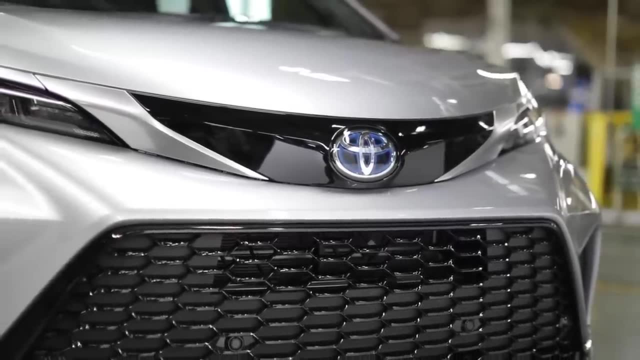 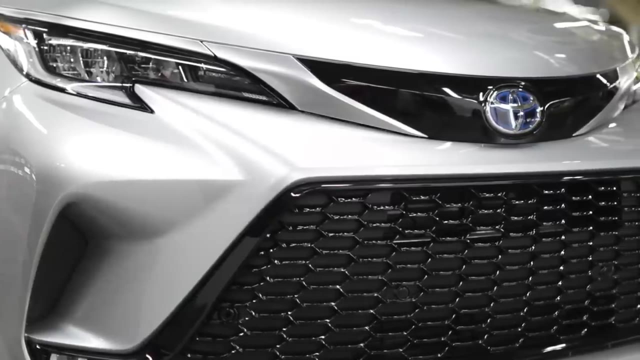 And that is something of interest, because perhaps here in North America people are beginning to realize that minivans can represent both brand recognition or luxury, comfort or even coolness. Elsewhere in the world it is definitely becoming more trendy. So even though this Sienna right here might not be the most trendy vehicle to drive around, 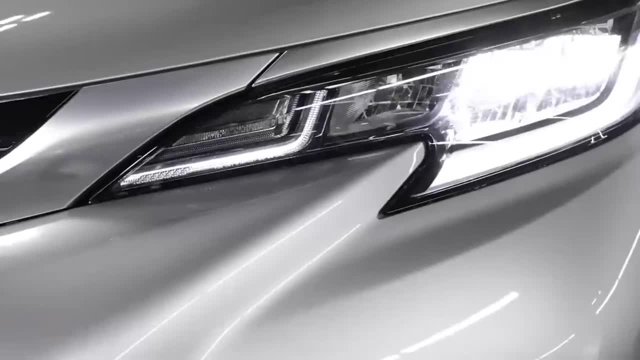 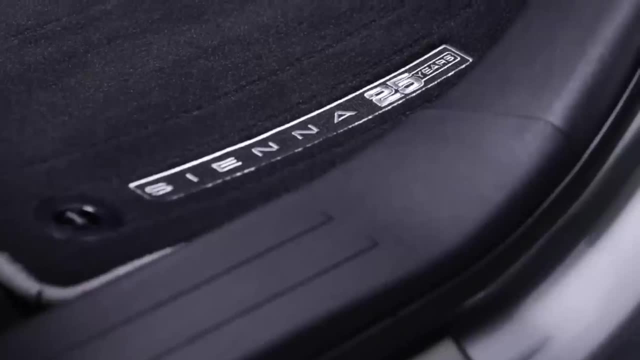 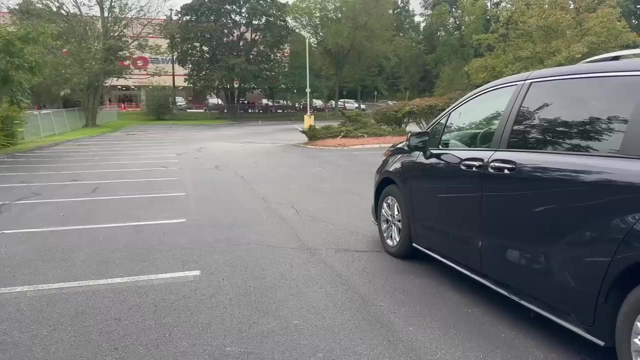 you know what? it could be very different in a few years time if Lexus introduces something like an LM to the market and everybody's going to begin to think that minivans can offer luxury and can offer a cool factor. The last and the seventh point I want to talk about in terms of why minivans are great buy. 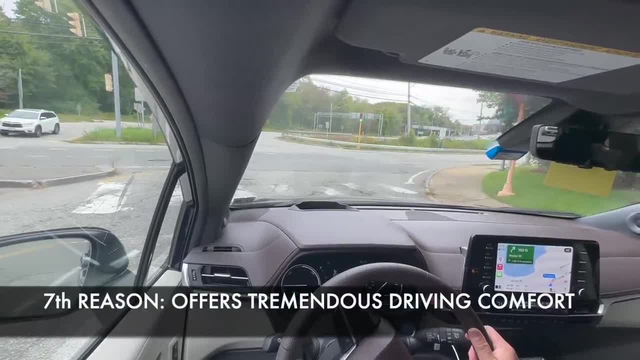 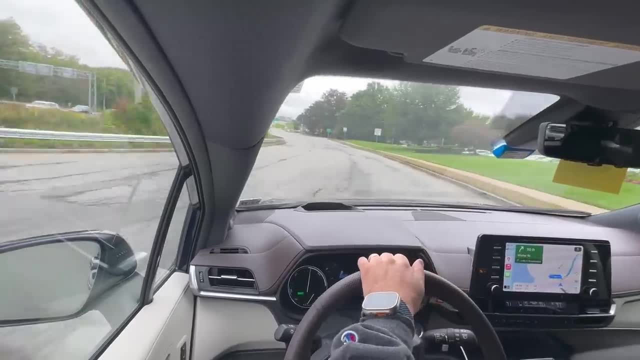 is the fact that it provides such amazing level of driving comfort- Maybe not so much for the driver, but at least for the passengers- in terms of quietness, refinement, smoothness, and then in terms of how the suspension is able to soak up bumpy. 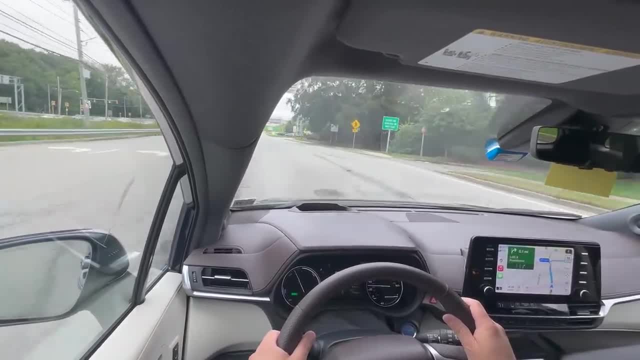 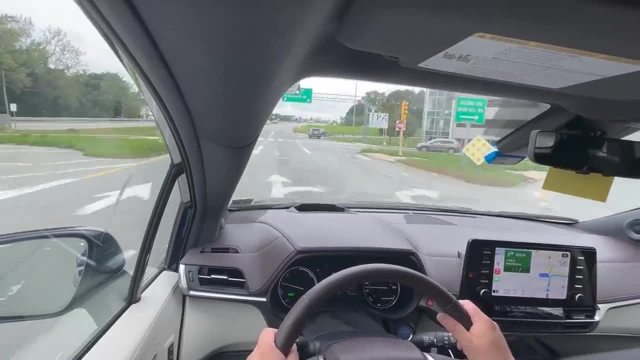 road. There's nothing that can beat minivans, because of the fact that minivans are a unitized body and then suspensions are calibrated for maximum comfort. All the passengers I have driven in minivans, like the Sienna, always say how comfortable. 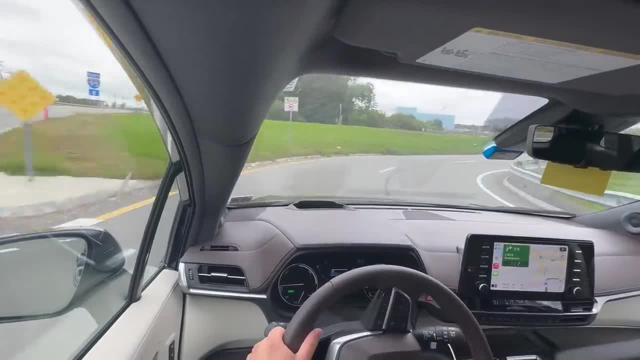 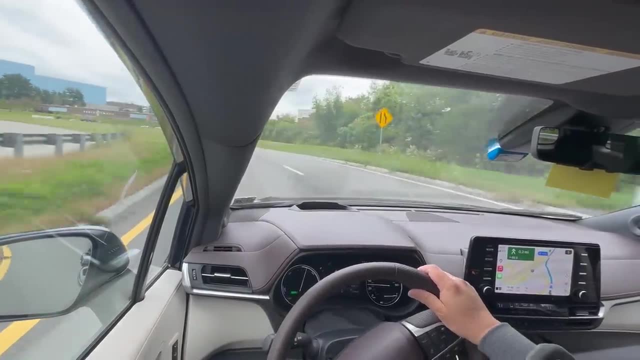 it is how quiet it is and how they can spend hours and hours in the minivan. Compare that to something like a Toyota Sequoia or a 4Runner or even the Lexus GX I'm driving- and you'll quickly realize that the minivan provides a better, refined feel on the road.